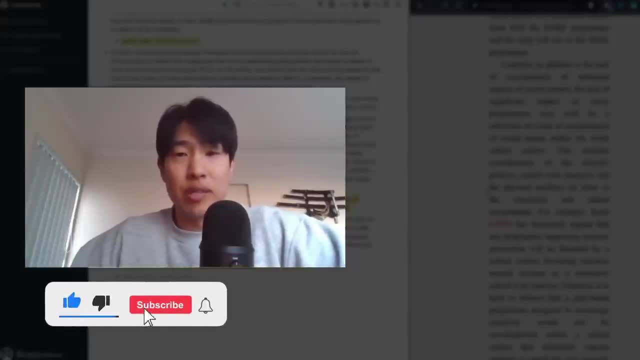 over and, over and over again, wasting my time and then getting progressively more tired. For those of you that don't know me, I'm Dr Justin. I'm a medical doctor and a learning and productivity coach. Now I know that I'm going to have to do a lot of reading and I'm going to have to focus. 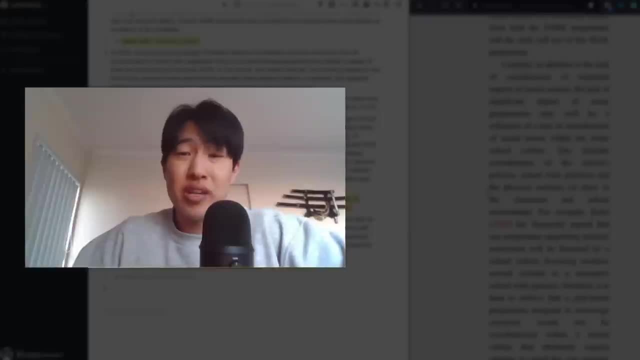 in a lot. If there's anything that's going to waste time in this process, which is already going to take me several hours, it's going to be losing focus and having to re-read sections. In fact, if you time yourself for, let's say, 20 or 30 minutes, you might find that half or more of 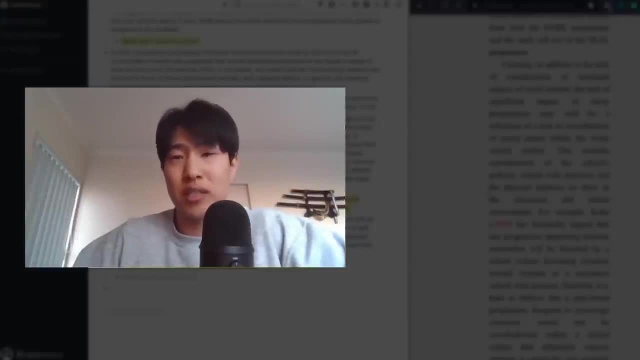 that time is actually spent on just trying to regain your focus, which is actually very frustrating. One of the things about reading quickly is that there is a technique to reading quickly and then there is a strategy to reading quickly, And the technique of reading quickly ends up being actually less important than the strategy when it comes to more. 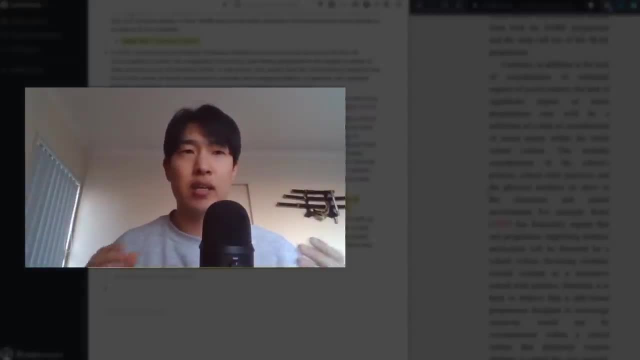 difficult texts. So, for example, if you're reading a easy like year four, year five, like a children's book, then your reading technique is the thing that is probably the most limiting step for you, because the time it takes to process the information is low. 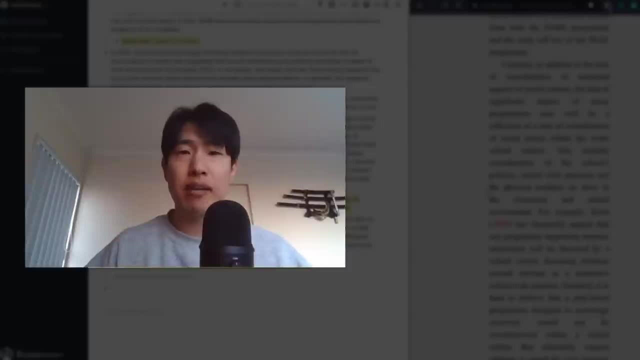 They're basic sentences with basic syntax and the information is clear and obvious and almost a little bit intuitive. So if you're reading a book, you're going to have to re-read it And when we know what to expect from what we're reading and if it's predictable and if the 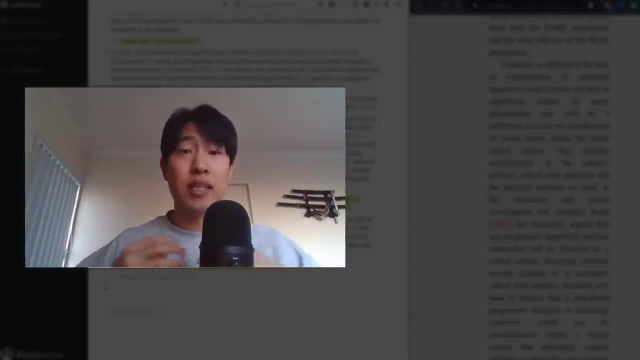 information is simple. if the words that are used are small, then it's much easier for our brain to process this, And this is, you know, relatively obvious. The thing that I have a problem with is that a lot of people will teach students that are trying to read textbooks that are much more. 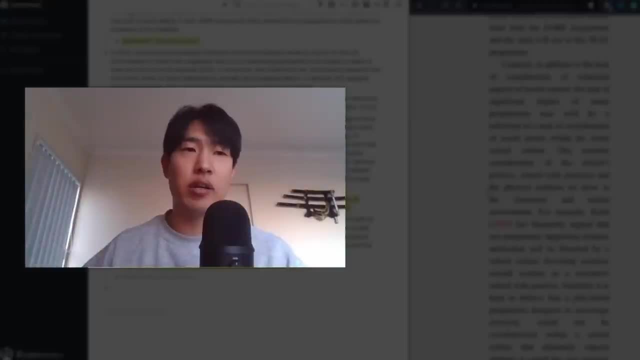 advanced and they'll teach them to read faster, relying on the reading technique rather than the reading strategy. And the thing is that at a certain point, the importance of technique actually drops by a lot, because the time it takes to actually process information gets longer and longer and longer, to the point where it doesn't really matter how fast or slow. 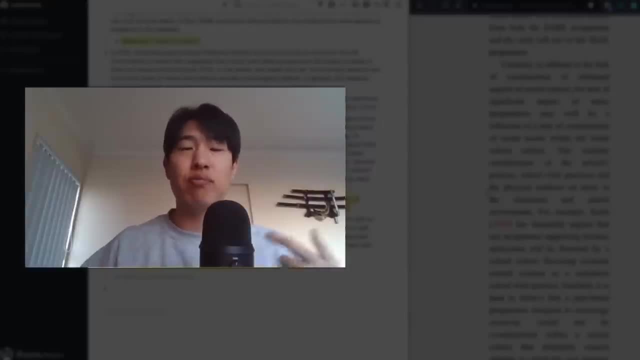 you're reading. The thing that actually makes the biggest difference is: how long does it take for your brain to kind of figure out what's going on, piece it all together, and how long can you actually maintain that concentration for? Because piecing things together is a more energy-consuming. 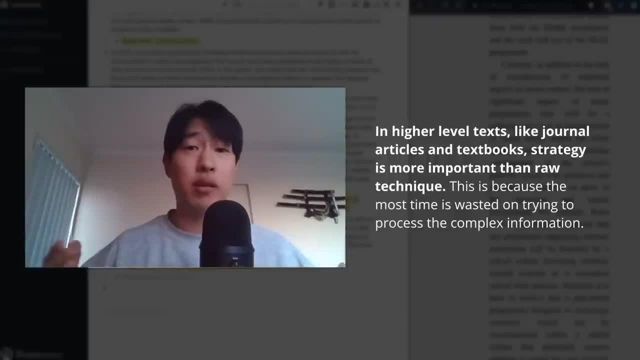 process, And so a lot of people can't speed read for more than a few minutes. So way back in 2009,, 2010,, when I first started looking into how to speed read, I got my reading speed pretty high- a thousand words per minute- but it was honestly quite unsustainable. I would be exhausted after. 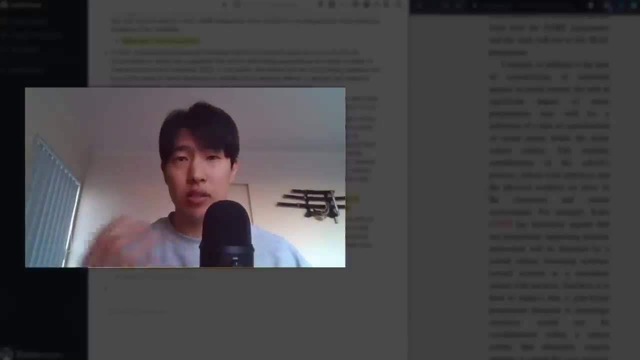 just a few minutes of reading at that speed And even though now I can still comfortably maintain it- you know, maintain a speed of around maybe five or 600 without having to concentrate too hard- I don't find myself resorting to those techniques as heavily as I thought I would going. 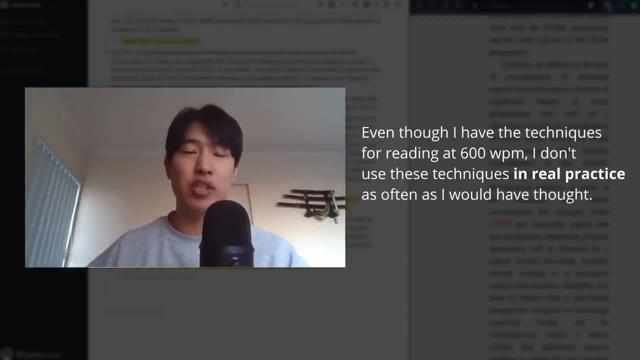 into it. Now. the biggest thing is actually about the strategy, So I'll cover some of the technique very briefly, just so that you're aware, because it does help, but then I'll talk more about the strategy and how you can structure your learning and set things up to make it easier So you can. 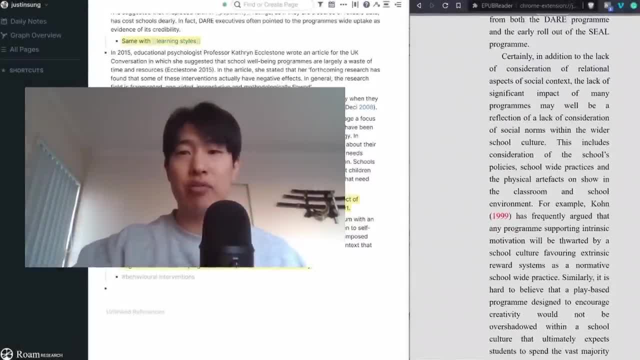 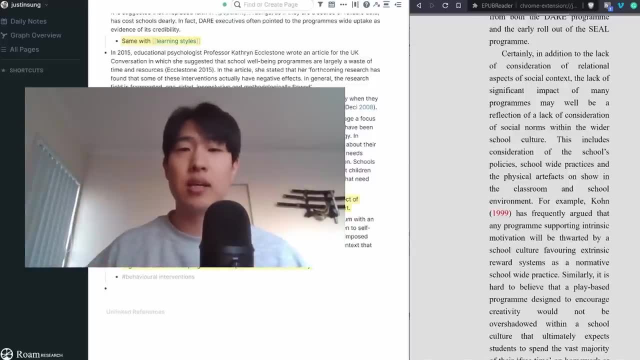 see that I've got some text here that I'm going to be reading through and I'm demonstrating, and you'll probably notice already a few things about how I've laid out this text. And if you're really interested to know about my app stacks, then leave a comment and I might do a video on. 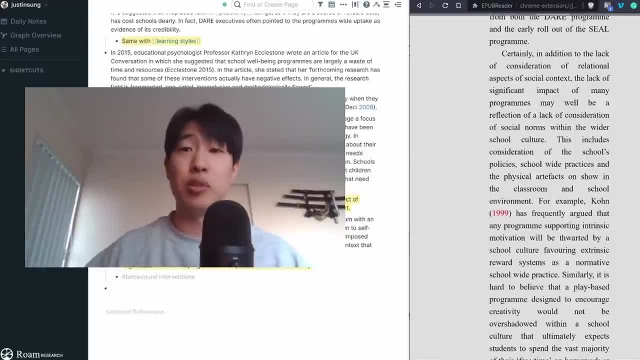 that too. You'll find that my app stack is actually really simple. It used to be a really super complicated, but I got rid of really a lot of those apps that weren't doing much, So the technology I use to facilitate my learning is actually surprisingly very minimal. So, in terms 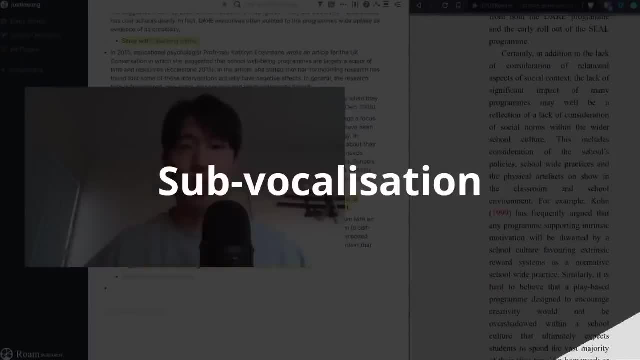 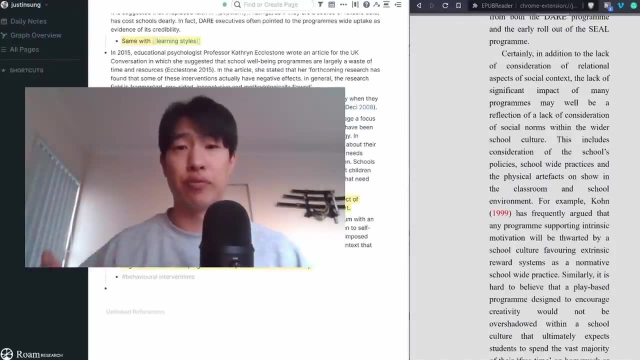 of reading technique. one of the things that's often talked about is reducing what's called sub-vocalization. So vocalization is what I'm doing right now. I'm just talking. Sub-vocalization exists in a couple of different forms. A very beginner level of sub-vocalization is actually 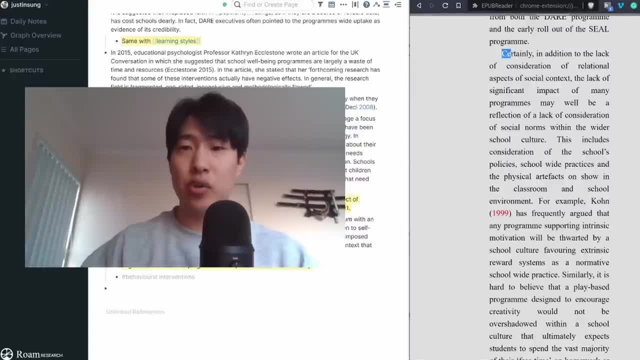 muttering the words out loud. So if we were to take this sentence right here, it says: certainly blah blah, blah, blah. Sub-vocalizing might sound like this, Certainly in addition to the lack of consideration of relational aspects of social context. 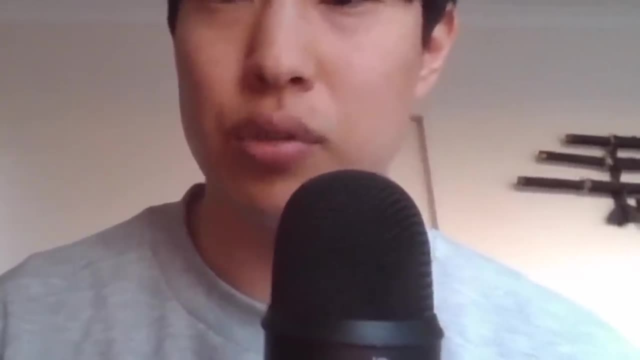 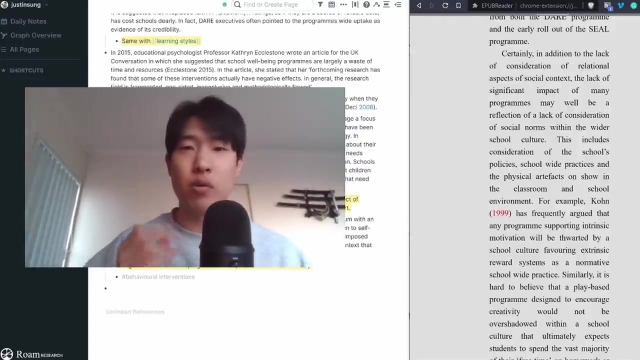 the lack of significant impact of many programs will be a reflection of a lack of consideration of social norms within the wider school culture. Okay, So what I'm doing now is I'm not really enunciating the words properly and I'm not taking time to really vocalize it properly. 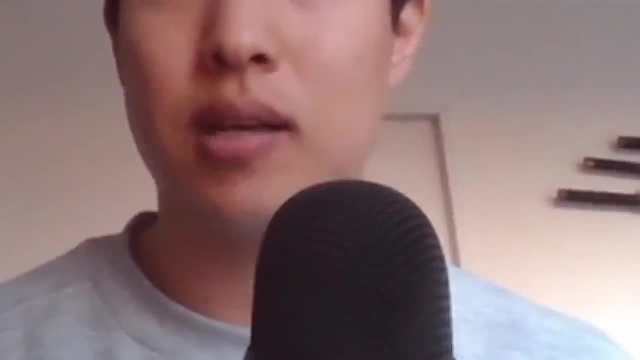 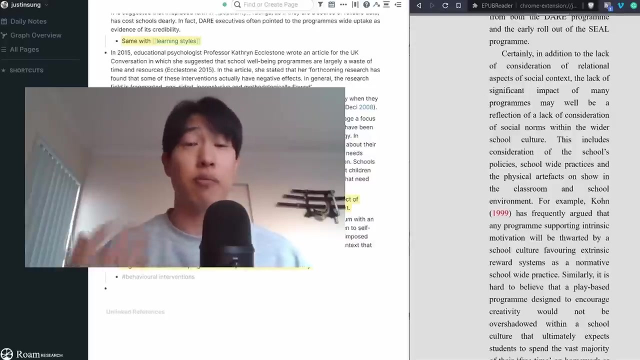 but I am sort of mouthing the words and it can be silent, just essentially reading it, but quietly and very, very quickly. And so the time save of not vocalizing instead of just sub-vocalizing is that we don't have to wait. 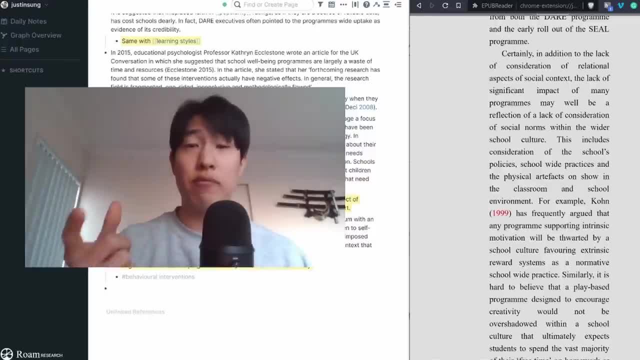 For us to properly form the words And so we can read a little bit faster. And so, straight away from going from vocalization to sub-vocalization, you will have a speed increase of maybe 10 to 20%. However, most people are already able to not need to read through vocalization. The next level of 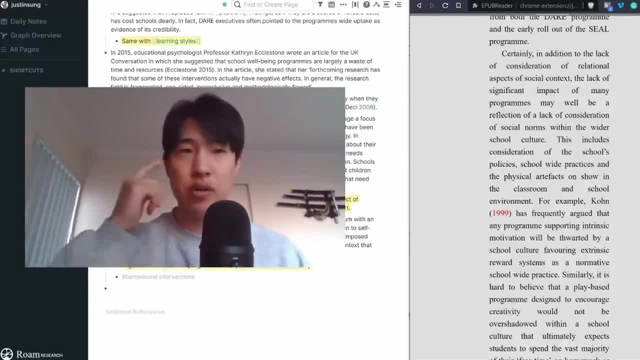 sub-vocalization is: your mouth is not moving, but you're still reading it inside your brain. So your mind is reading it silently. So on the outside it doesn't look any different, But in my head I'm still kind of reading it. So I'm doing the same sub-vocalization that I was. 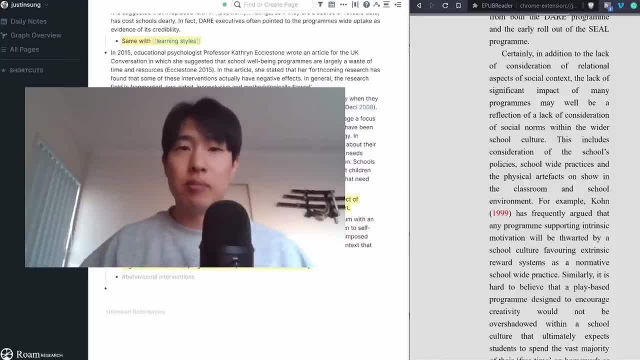 doing My mouth, but I'm doing it in my brain. Now that's a little bit faster still, because I don't have to even wait for my mouth to kind of mutter everything out. However, that does put a hard cap on how fast that you can read A lot of techniques around reading technique and speed. 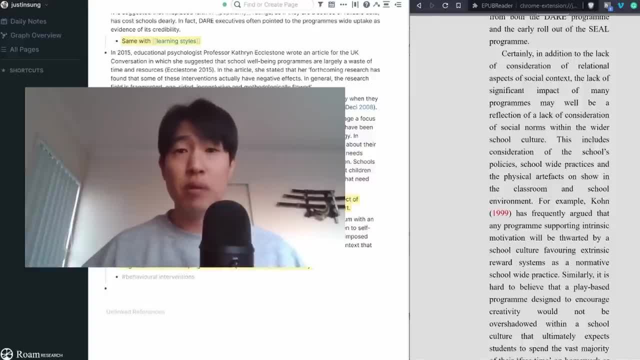 reading, focus on how to reduce sub-vocalization. The problem is, though, sub-vocalization is also associated with easier processing, So it reduces what's known as cognitive load and allows it to be a little bit more manageable. So when you're reading, it's easier to process the information by sub-vocalizing. So sub-vocalizing. 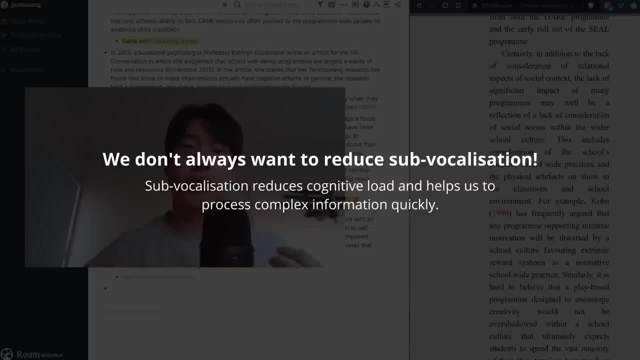 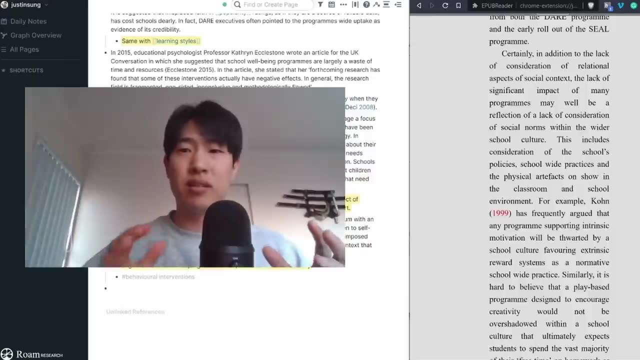 isn't necessarily a negative thing. It does make you slower, but it also makes it easier to process information. So sub-vocalization is actually a strategy that we want to use. We don't want to sub-vocalize when the text is not very important, but we want to sub-vocalize in areas where we know. 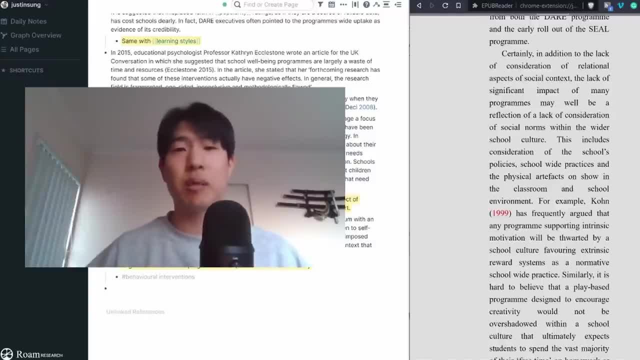 it's more dense to process because, trying to process it without sub-vocalization, you may be able to read the words faster, but it would actually take you longer to learn from it, Which means that you might end up having to reread the same thing three or four times And then on the 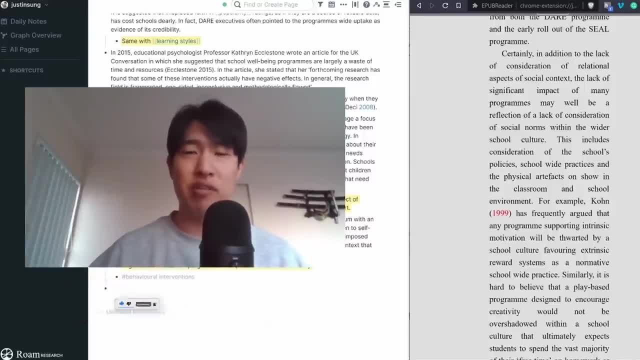 fourth time. you probably end up sub-vocalizing it anyway, because you're just frustrated from having to reread it so much. And all of this wastes energy and it reduces your focus. So, sub-vocalization: we want to learn how we can turn it off, but we also want to know that we it's not necessarily a bad. 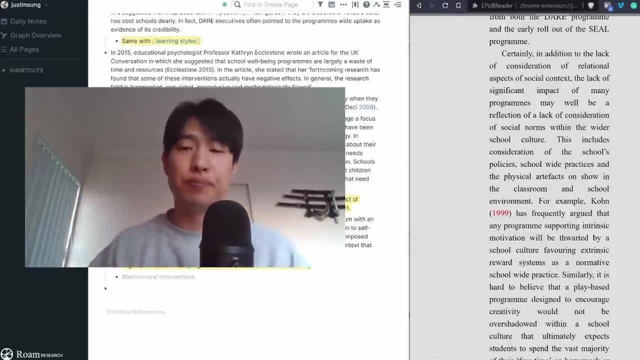 thing. We want to be able to use it when we can, And that's part of the strategy that I'll talk about soon. How do you turn it off? Well, there's a number of different ways, Some people will say, to hum in your mind as you're doing, or you can hum out loud as you're doing it, just as you're doing it. 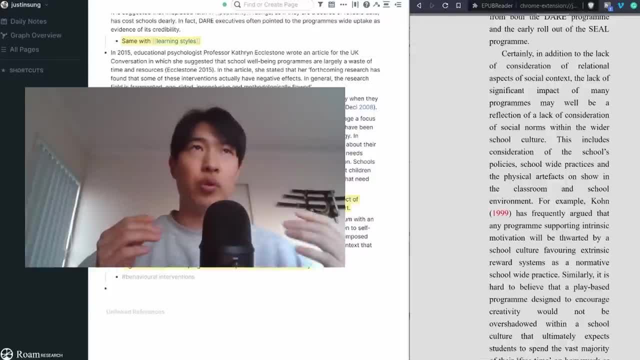 Imagining sort of silence or trying to sort of count or something while you like in your head, while you're reading. Personally, I find that maybe the only thing that really works there is the humming in your mind, but I don't find that that is a very effective way of training sub-vocalization. 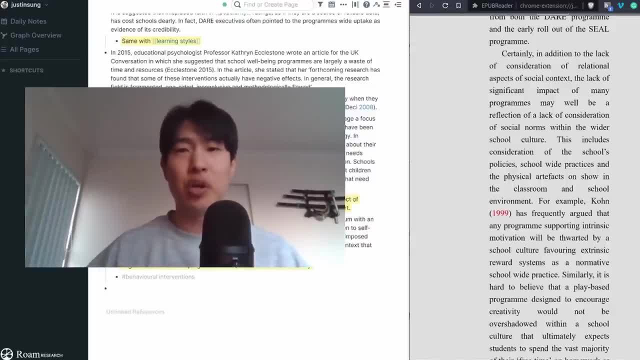 And I trained that for about a week or so, 10 plus years ago, when I first got into this, And I found it to be number one, a very boring, but number two, not a very sustainable way of practicing. And you don't actually need to do that, because there's another aspect of reading technique that 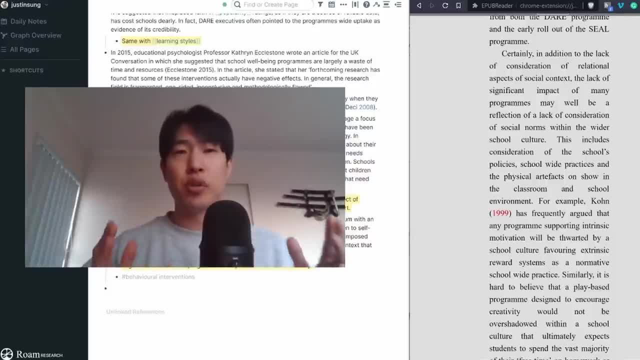 is actually more important, which is grouping words together. So your eye, when you're looking at something, has the ability, obviously, to see more than just like a single point. you know, There's a certain width at which your eye is able to look And this width is actually defined by 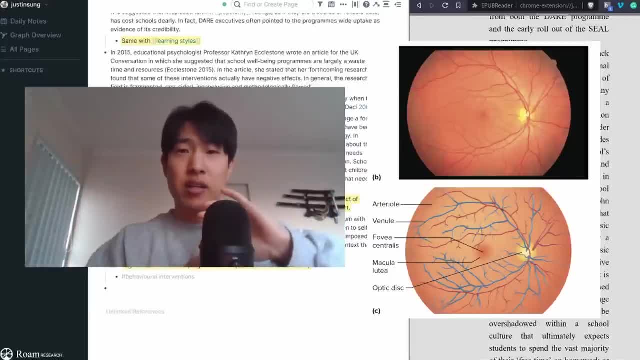 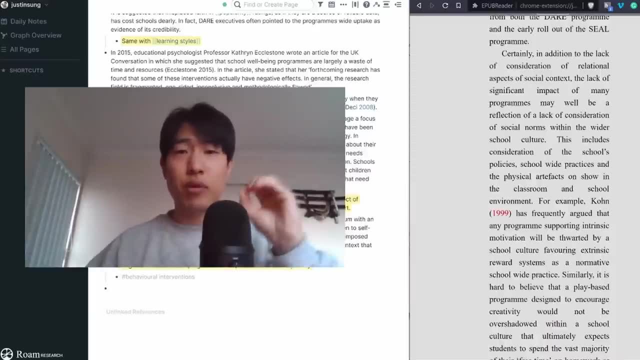 a area on the back of your eye, on the retina, which is especially dense and has a lot of, basically, nerve fibers that detect light and can process it. Light that is centered right there, which is right in the center of your vision, is processed much more and much more information. 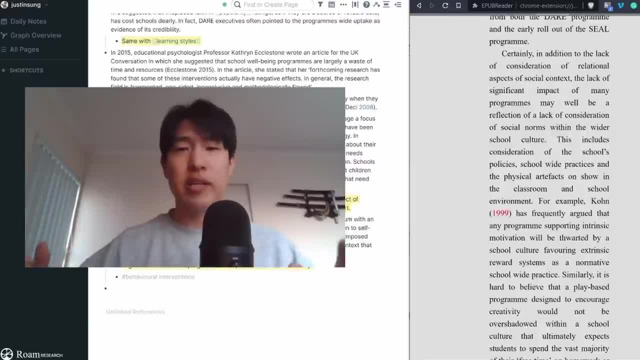 comes in. That's why your peripheral vision is usually much blurrier and you can't really focus on anything more than just like a very narrow cone within your central vision. What often happens when we are reading is that we are really, really intense with our reading. And then what that? 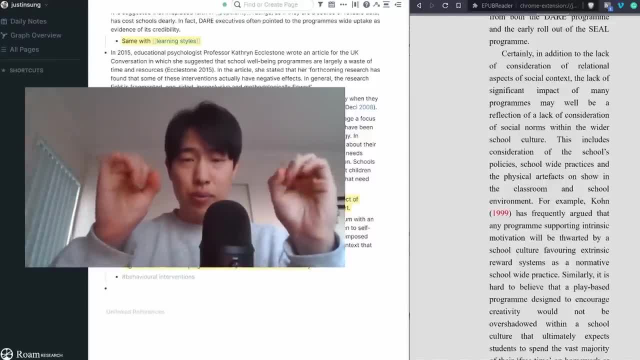 causes is a constriction of our pupils, which makes it so that that cone gets even narrower. What we want to do is we want to be a little bit more more relaxed. by relaxing our eyes a little bit more, that pupil enlarges a little bit more and 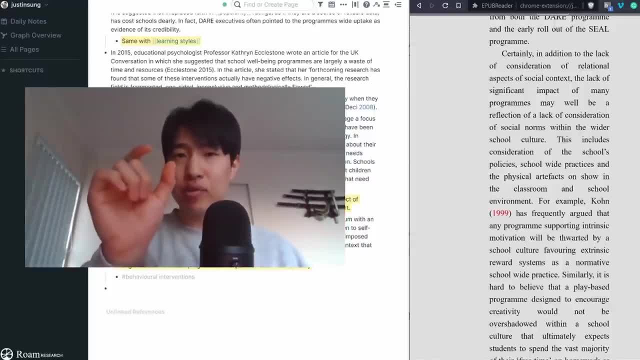 allows a little bit more light to come in, And so it just increases that peripheral vision just by a touch- not by much, but just a little bit. And when you read a little bit more relaxed, you'll be able to find that you're able to see a few more words at the same time. So instead of reading this, 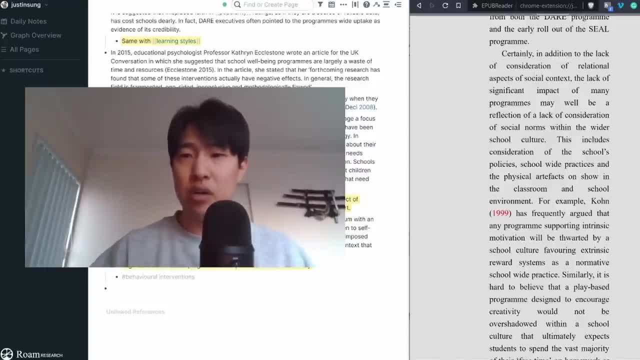 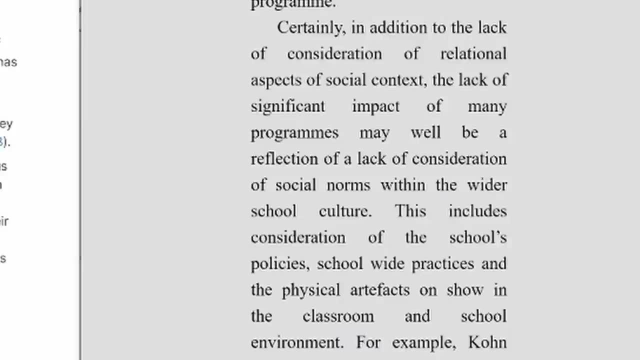 paragraph certainly, in addition to the lack of consideration of relational aspects of social context. I would read this: potentially, if I'm just starting out, I would put my eye relaxedly in the middle between the words certainly and in, and then I'd be able to. 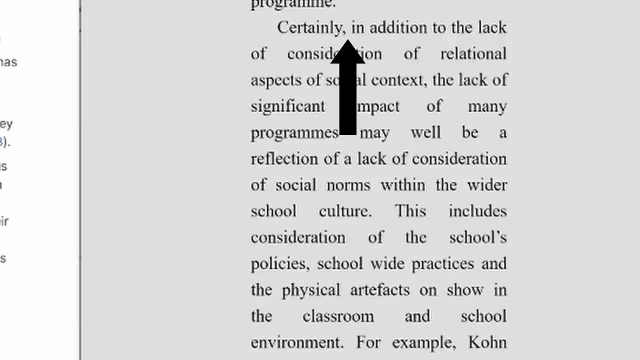 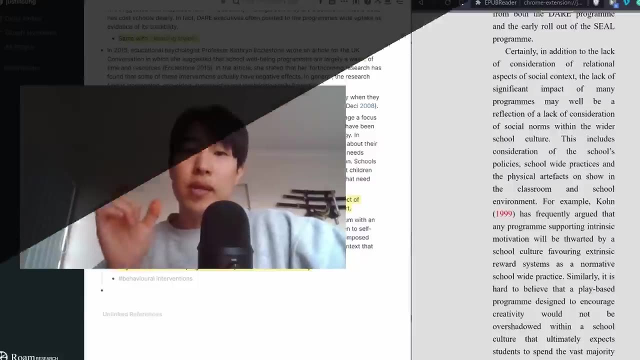 in a single go. read both words, certainly in, and then I'd be able to read addition to, and then the lack. So by putting my eye here, here and then here, I'm able to read six words with three different eye positions. and grouping words automatically shuts off sub vocalization. 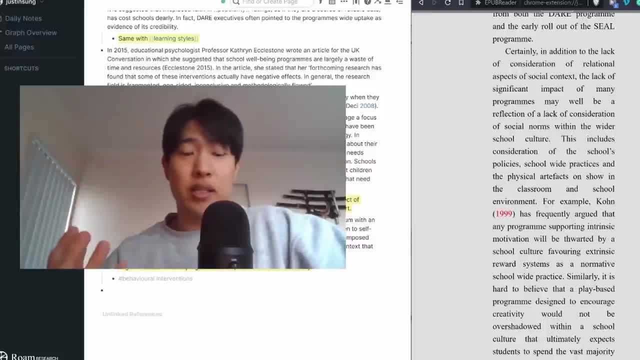 because you can't pronounce two words simultaneously in your mind. We're turning off sub vocalization, while we are reducing the amount of words that we need to read by grouping the words together. Grouping words is also more energy efficient, So instead of just going through and reading every 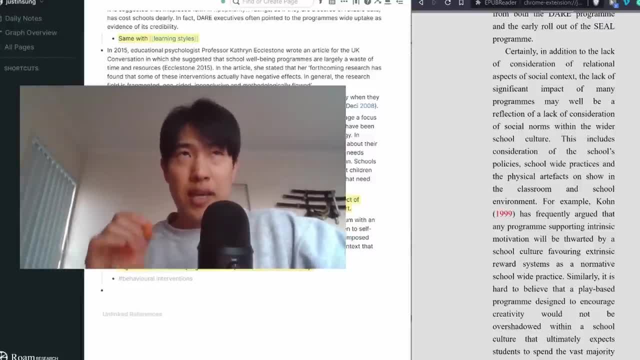 single word. when you group words, you can group. the words that you can tell are a little bit more difficult to process. A very easy way of doing this is just the number of letters in the word. So I know that the word in to and the are words that are very easy to process. 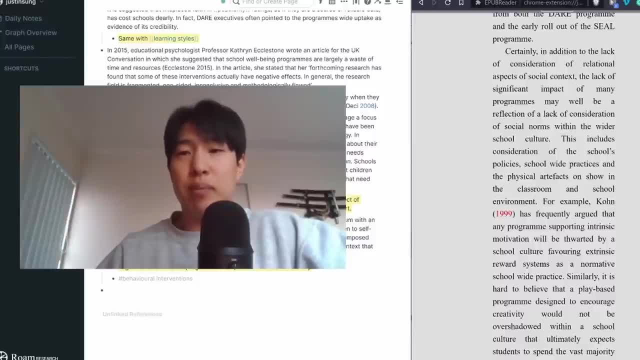 in fact I can read, certainly in addition, all at once by gently placing my eye here and boom, I can take in this group of words at the same time. Now it might take a little bit longer- 10% longer- to read a group of three words than it would to read a single word. So let's say it takes. 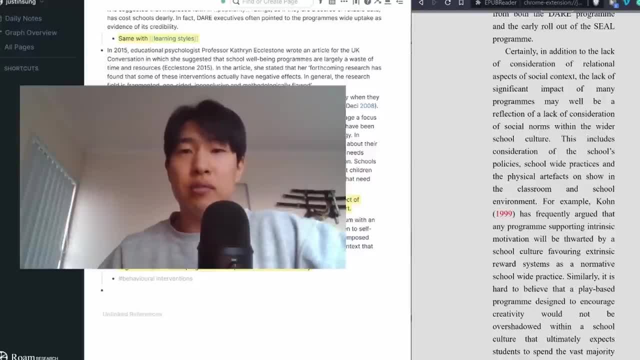 0.1 seconds to read the word Certainly. it might take 0.0, 0.15 seconds to read certainly in addition. So your eye is going to be moving slower, However, the amount of information you're taking in 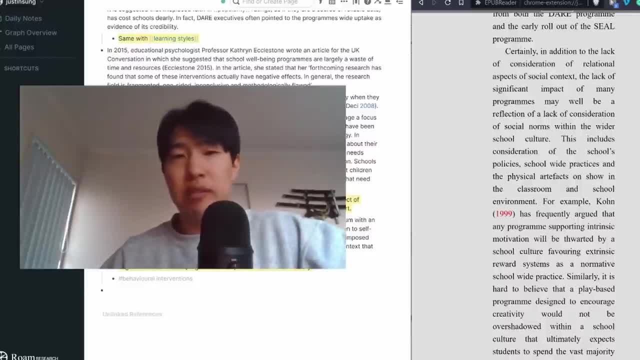 is actually faster. So just because you're grouping, let's say, three or four words together at a time, doesn't mean that your reading speed has increased by three to four times. It doesn't really scale that way, because your eye is not moving at that same speed. Instead, if you're 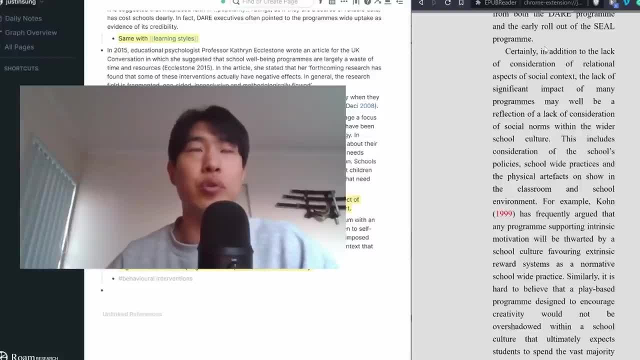 grouping three or four words at the same time, you may be able to increase your reading speed by maybe 60 or 70 or 80%. So grouping words together is actually probably the most time efficient, energy efficient and practically useful technique when it comes to. 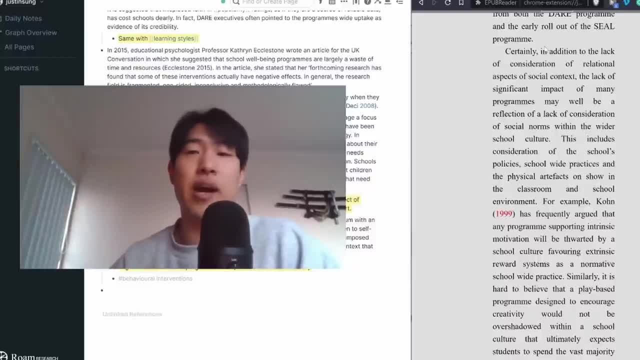 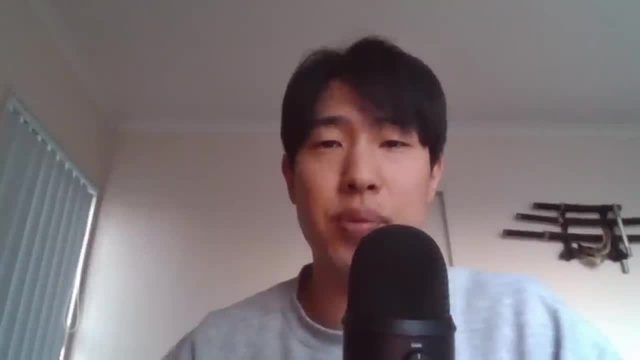 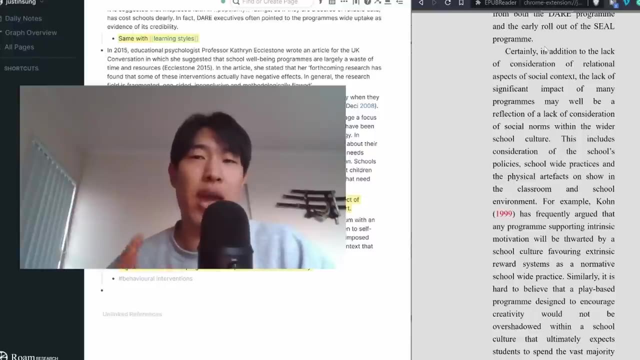 speed reading high level academic texts like you'd find in a textbook. Personally, as someone that does really a lot of reading on a daily and weekly basis, grouping is the only actual reading technique that I use or rely on. It's very rare for me to actively think about turning off sub vocalization. 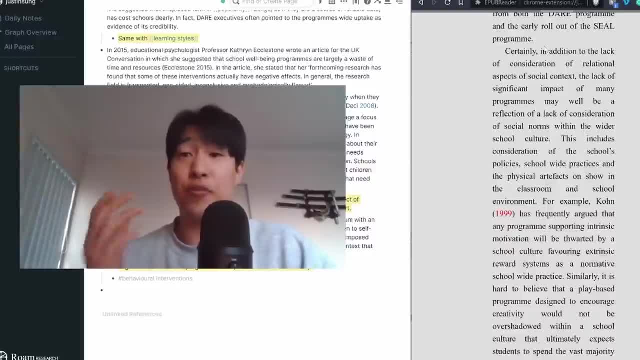 When I group words together, sub vocalization turns off automatically. If you're first starting out on this, you will need to practice. You may need to practice for a few hours to really get the hang of it, But once you get the hang of it it just becomes an automatic thing and your brain 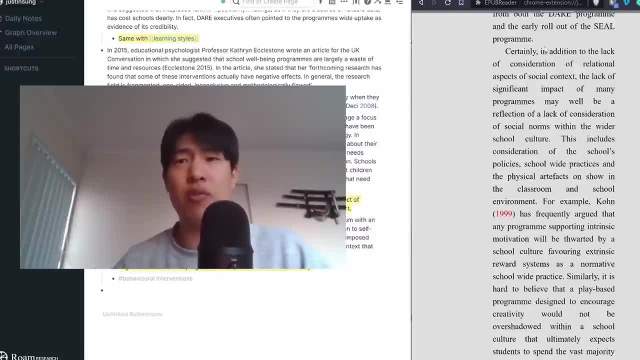 just gets better and better at it. Now, this is really only for nonfiction books. by the way, If you're reading a fiction book, yeah, sub vocalize whatever you want to do. Read word for word, for word. You want to immerse yourself in the story. This is really just when your goal is rapid. 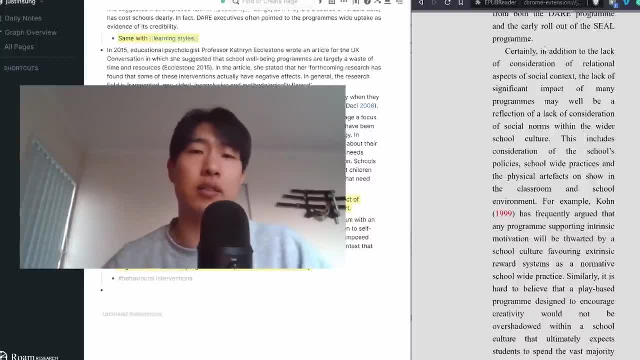 information consumption. So that's the reading technique side of things- is that we're grouping the words together. The strategy comes from when we use that technique. So ideally, what we want to do is we want to be able to skip through the information that is not very meaningful. 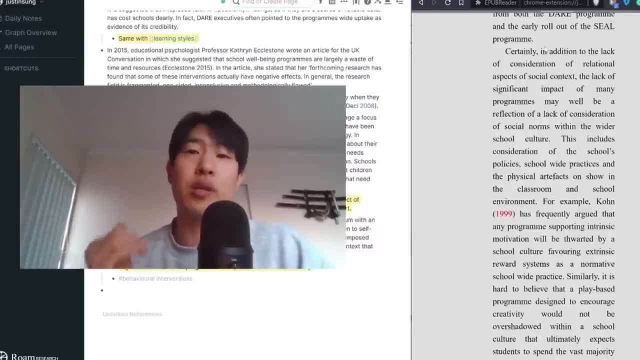 and we want to sub vocalize on the areas that we know are the most difficult. So what that means is that we're saving energy where we don't need to be thinking so hard, And then we're using that energy in a productive way to get maximum learning, And we're actually using sub vocalization. 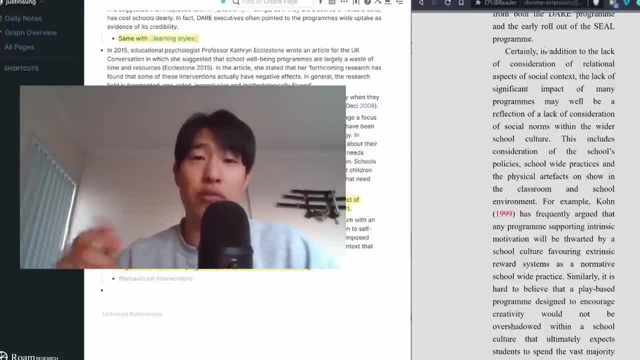 as a tool. So all we do there is we turn on and off the grouping. So, for example, if I'm going through this text, I can, without even reading it, tell that there are certain aspects of this text that are going to be a little bit denser based on the amount of big words that are coming up. So 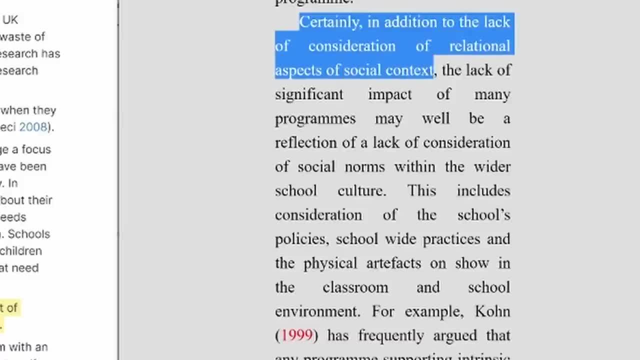 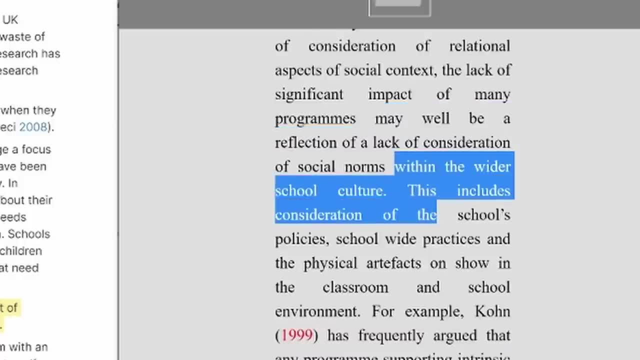 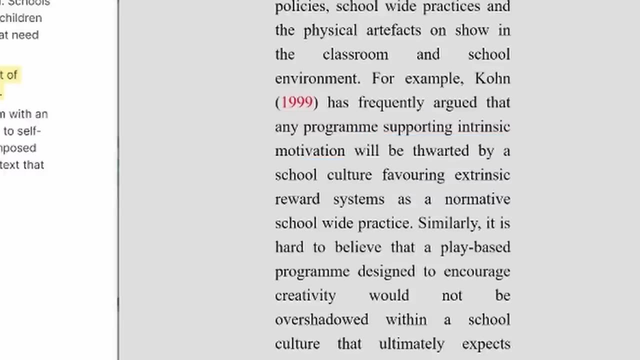 for example, I can tell that maybe this area here is a little bit denser, But for example, maybe this area seems a little bit easier, This area seems a little bit easier, This seems a little bit easier, This seems a little bit easier. So you can see, there are little pockets where I can. 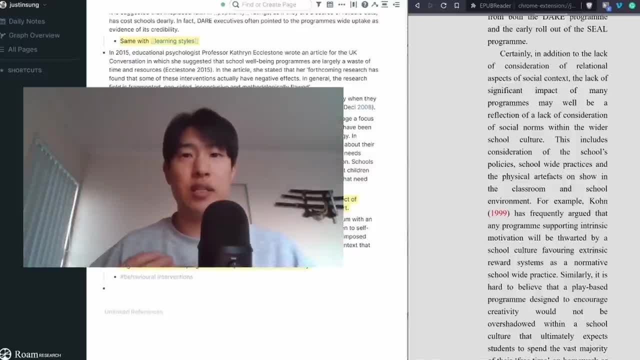 group, And this is very important. So you should be reading in these very discreet, concentrated bursts of speed. you're rapidly sprinting from point to point to point. The other part of the strategy is that you need to give yourself sufficient pause. 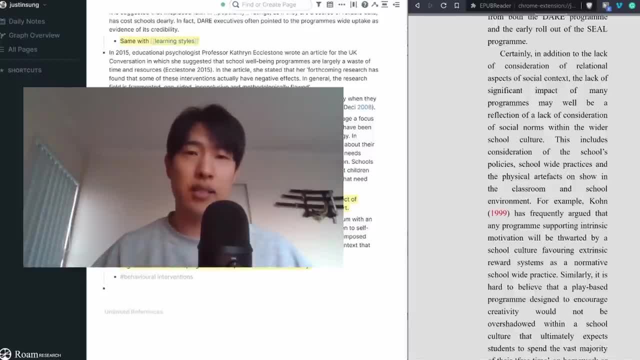 As I mentioned early on, one of the biggest things that's going to hold you back is actually how long it takes for you to process the information, as well as how tired you get and how long you can sustain that, for There's no point being able to read it: 1000 words per minute, But then five. 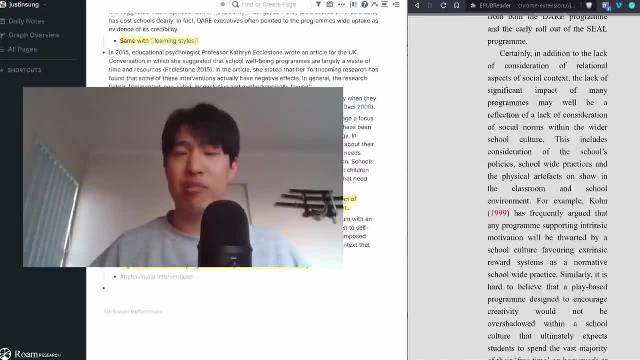 minutes later you need to take a 15 minute rest. you may as well have read at 300 words per minute, but then still be energetic enough to go for an additional three or four minutes, And then you would have actually read and consumed more in the amount of time. 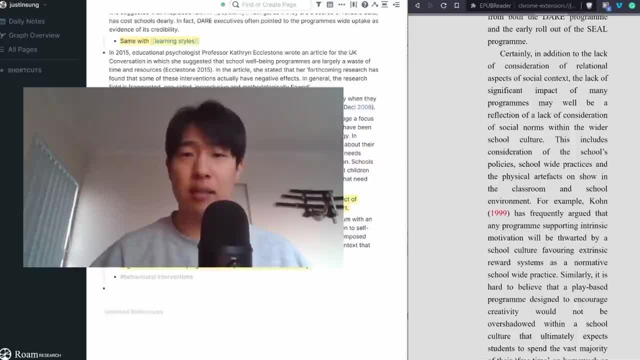 So taking strategic processing breaks and pauses is an important part of the technique. What that means is that between my sprints of reading I'm going to stop, pause, think about what it is that I've just read, kind of make a mental log of kind of what's going on And the important thing- 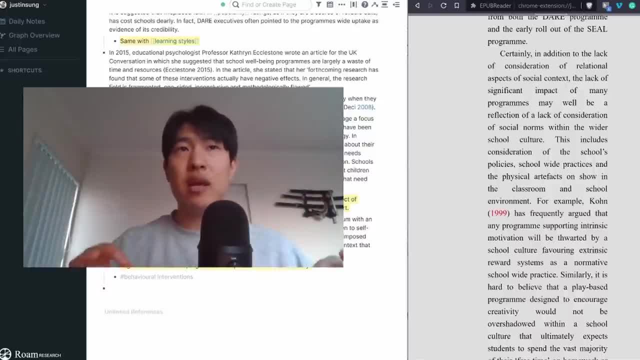 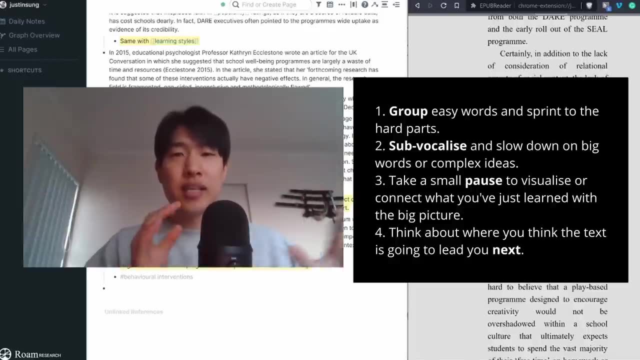 is spend maybe three or four seconds kind of thinking about where this text is likely to take me. I'm kind of trying to predict where this text is going and what information I'm going to consume. So you remember when I said that reading a really easy book makes it easy to read, because 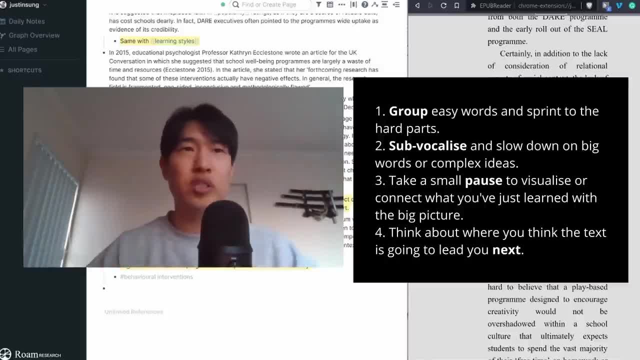 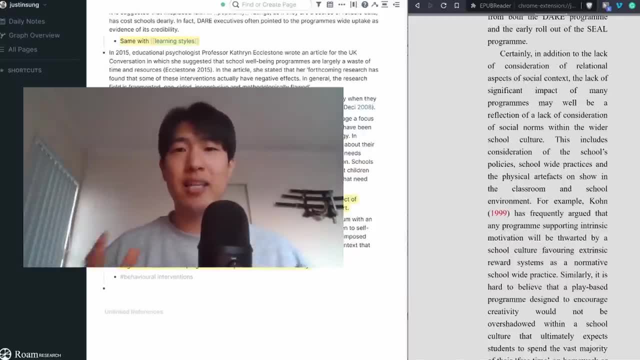 it's predictable, The sentence is predictable, the story is predictable. the words that are used are not particularly fancy. It's easy, because your mind can already kind of guess what's going to come next. In highly academic text, the processing time is often so long that it's right up against. 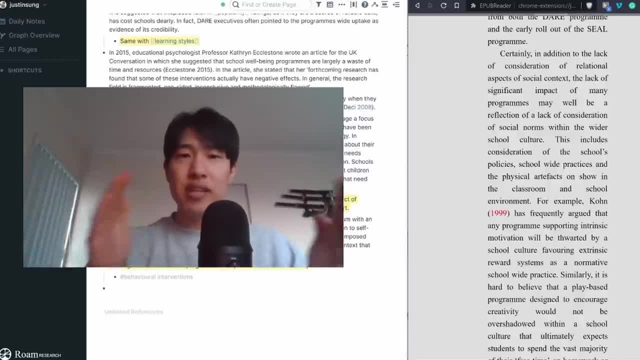 the reading time. So every word you read is being processed. So you're never really giving your brain enough space to think ahead of where your reading is, to get an idea about what might be coming next. Taking these processing breaks gives you the ability to just think about what. 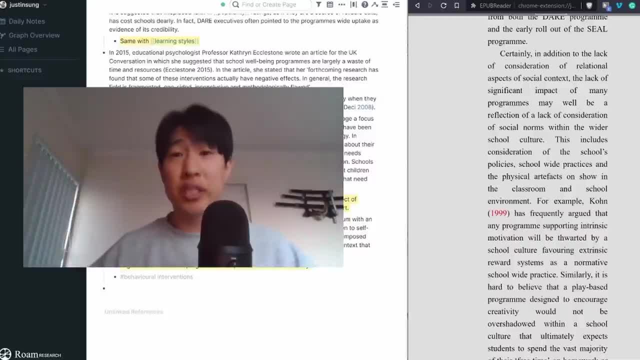 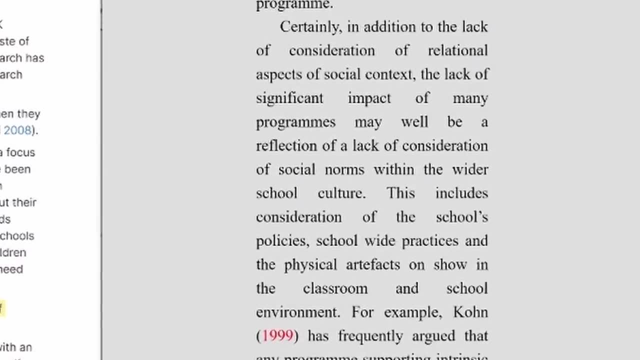 might be coming next And you'll find that that makes reading it actually much easier and much smoother and much more effortless. So what that might look like is, when I'm reading, just going through and saying, okay, so I'm going to read through this block, starting from here down. 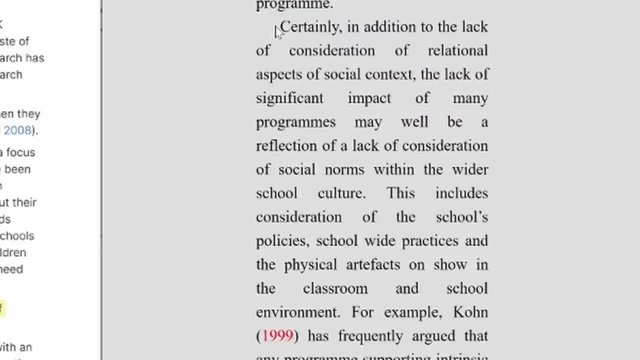 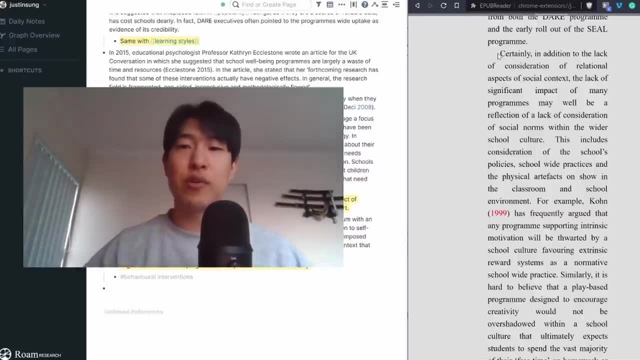 and I'll just start now And I'm going to be grouping and sprinting and sub-vocalizing wherever I need to, And what I will do is I will show you how I'm doing this with literal examples. Instead of sub-vocalizing it in my mind, I will sub-vocalize it out loud, So that means that you can see when. 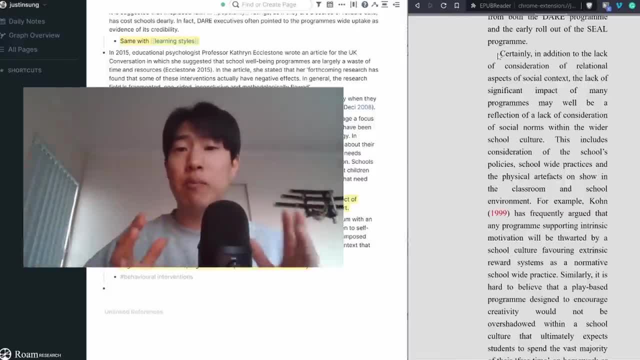 I'm grouping because I'll be silent, and then where I'm sub-vocalizing, because I will say it out loud into the mic And you can follow along with me to see that pattern of bursts And you'll find that the bursts are very short but they're very free And you can see that the bursts are. 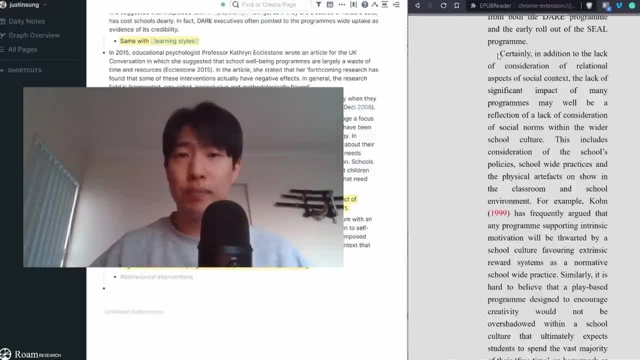 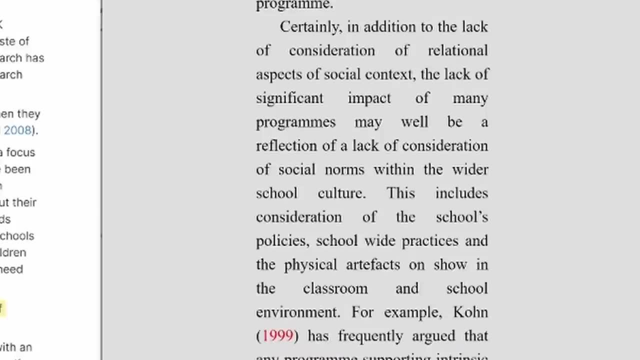 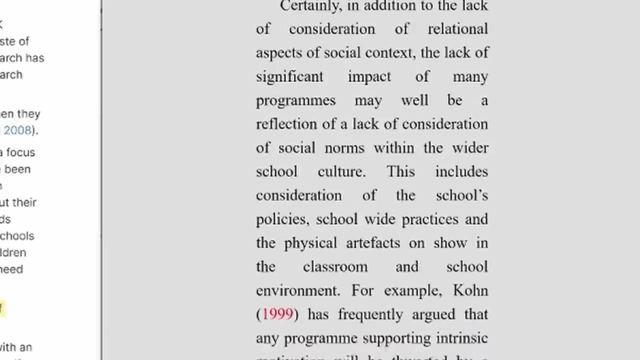 frequent And I want you to note when I'm doing my pause, So let me demonstrate Certainly. in addition, relational aspects of programs reflect consideration, norms, culture, Consideration of policies, practice artifacts, classrooms, school environment. Okay, so I've just read up to here. 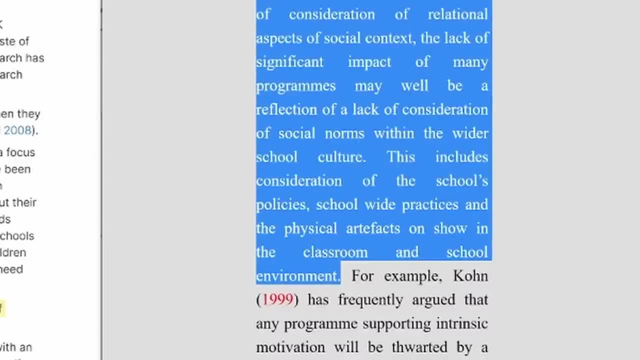 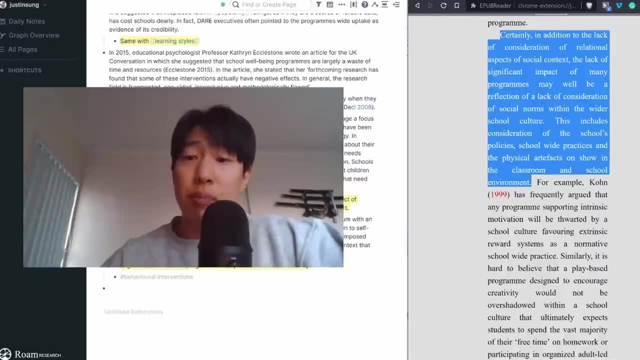 Okay, so you can see that I basically have grouped and then sub-vocalized individual kind of key words within that and I'm piecing it together Now at about this point because my reading speed is relatively fast- at about this point. 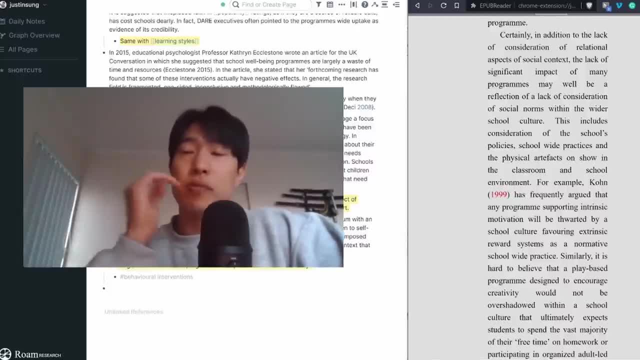 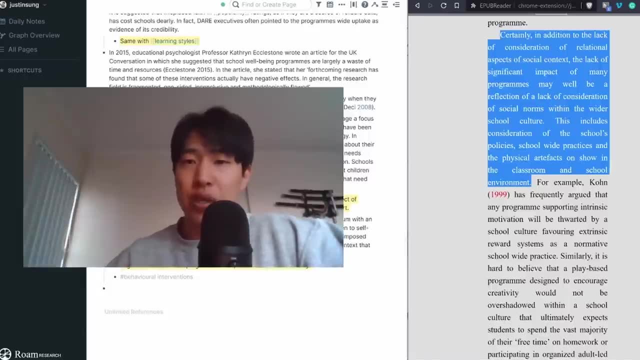 I'm just going to take my break And I'm just going to think about what I've just read. Cool, So I know that this paragraph- because you probably weren't following along- is talking about the different aspects of social and emotional learning and the programs that are used in school. 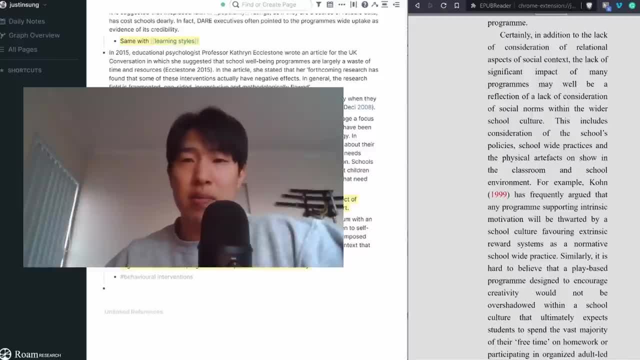 and the influence that different things like school culture and classroom environments can have on that. So I know that the next part of this article is probably going to give me well. I know that it says, for example, example of these wider influences, And then the rest of the narrative might talk a little bit. 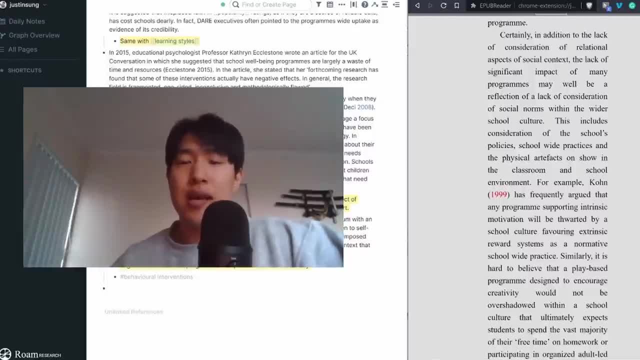 about different models or frameworks or pros and cons or benefits, And I'm expecting it to elaborate on that Very straightforward. I'm not making any crazy predictions or any crazy hypotheses. It's just maybe three or four or five seconds to just stop, think, understand, process. 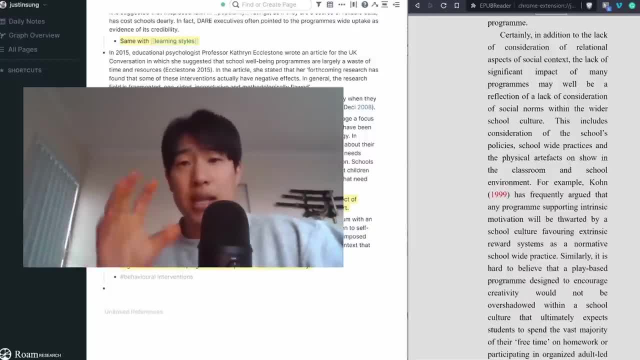 it Cool, Ready to move on, And you may want to write a few notes at that time as you go as well, using that break. But don't be afraid to take these breaks to really process it properly in order to move on If there. 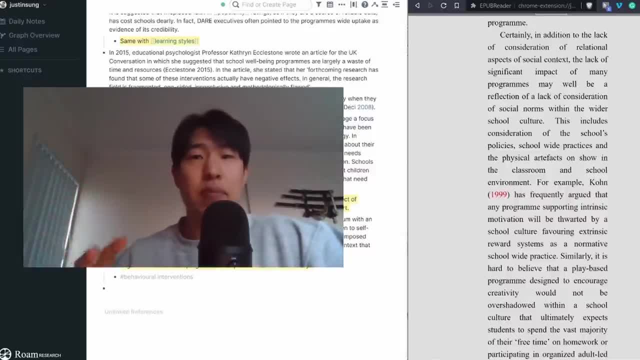 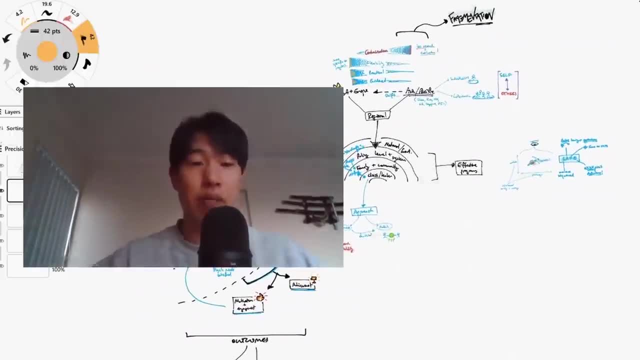 was something that was new in here that I really thought was conceptually important. I may make a reference to that in my room. depending on my workflow, If I'm studying, I may chuck it into my mind map. So every now and again I'll update my mind map as I go. Again, these are all techniques. 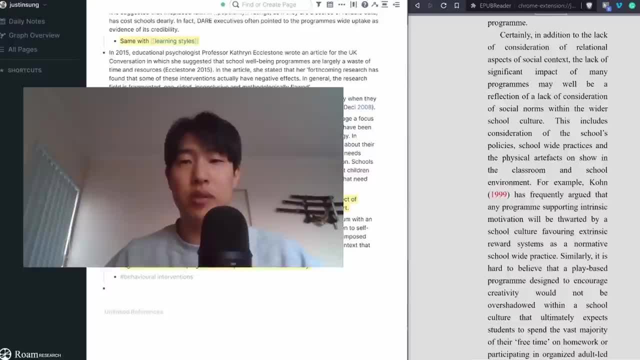 that I don't really have time to. Well, there's a lot of me right there. These are all techniques that I don't have time to really go into right now in this video, But you know, those of you that have been following my other videos- if you haven't done so, please do so, And if you haven't done so, 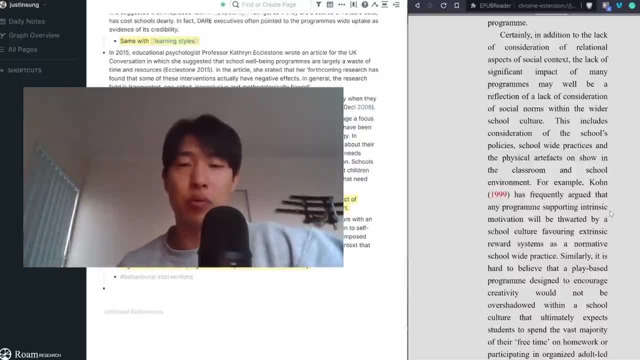 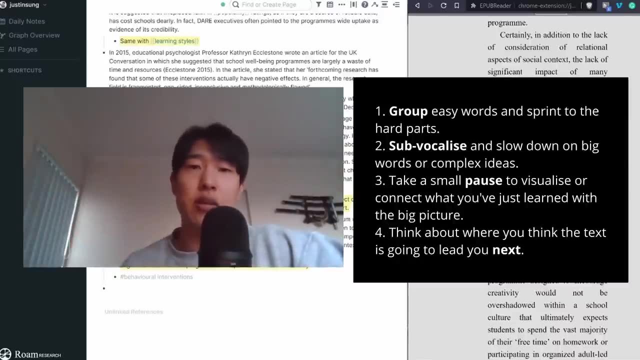 you'll see me demonstrate this multiple different times in multiple different contexts. So the final part of this. So we've covered the techniques, such as grouping the words together and using sub-vocalization strategically, and the strategy behind going in bursts, using and then not using. 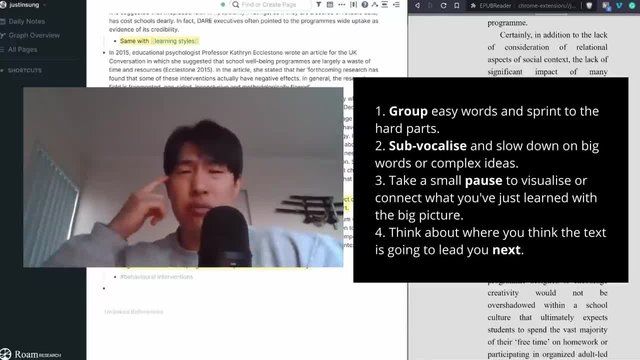 grouping of words. And again, if you're just starting, there's a lot of effort that goes into turning on and off grouping of words. But again you practice for a few hours and that'll become easier and easier and faster until you don't even have to think about it And then taking 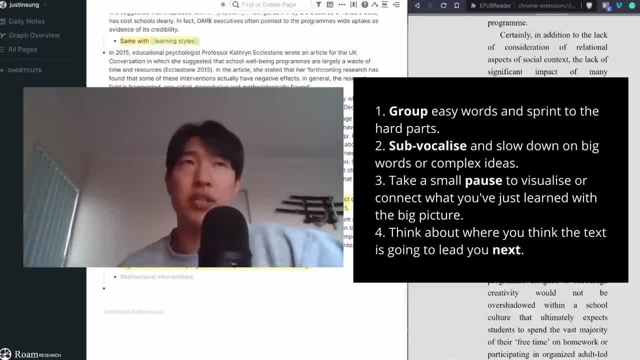 those processing breaks to really collect, process that information, make a few notes, whatever you want to do, and then just have a quick prediction about what's going to come next, And then that is actually going to reduce the amount of energy that you need to use. It's going to allow you to 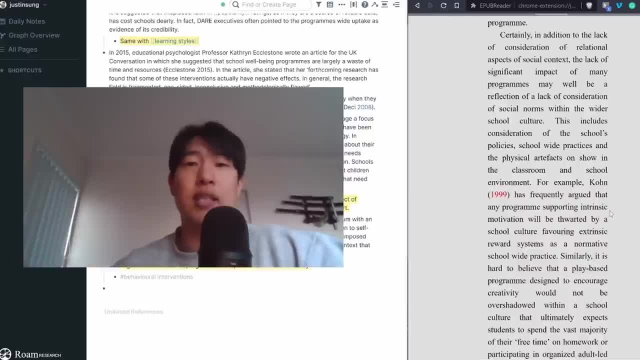 maintain a moderately high speed for a lot longer, And it's going to mean that your attention is actually really high going through it. So, using this technique, I can actually maintain this type of reading for several hours. In fact, I'm recording this video right now, but I've actually 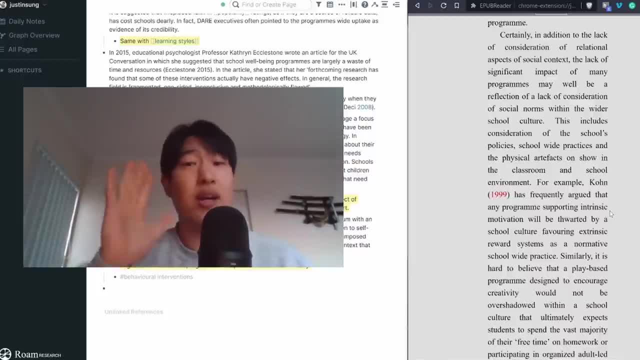 been reading for the last four and a half hours already. Now, tiny little tip- and I'm sure you've noticed- is just a little few technical things, If it is possible, and this is another reason I like using EPUB format is to make it a very 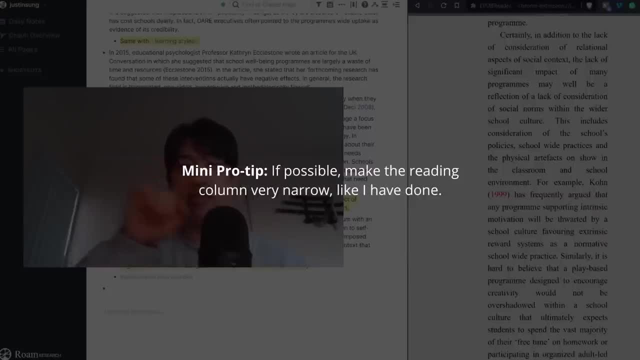 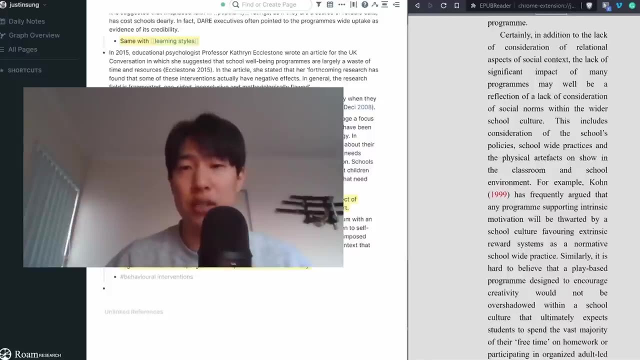 narrow field. So rather than moving your eye from left to right, left to right and down the page by grouping it like this, it allows me to read each line in just one or two eye positions. So instead of having to go imagine if the line was you know this long, instead of going one, 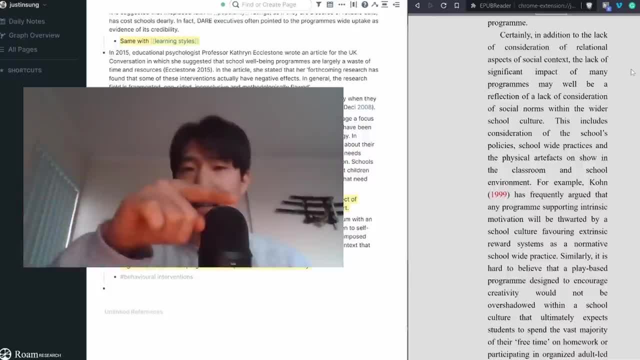 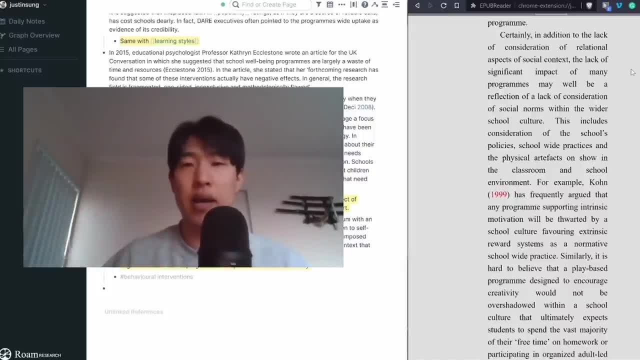 I'm scrolling more but it is easier on my eye. I'm not having to move my eye across like an entire screen or an entire page. I can generally keep my eye just between toggling between two general locations as I'm coming down, And these little little things just allow me to save a little bit. 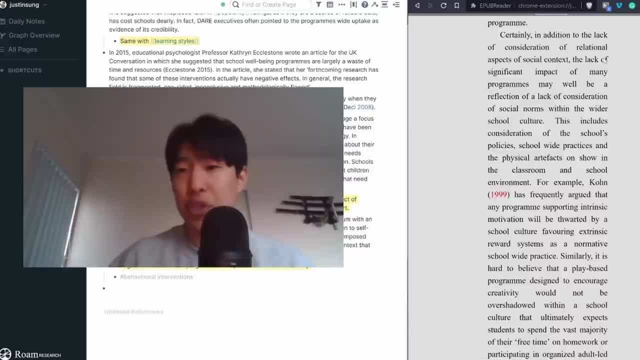 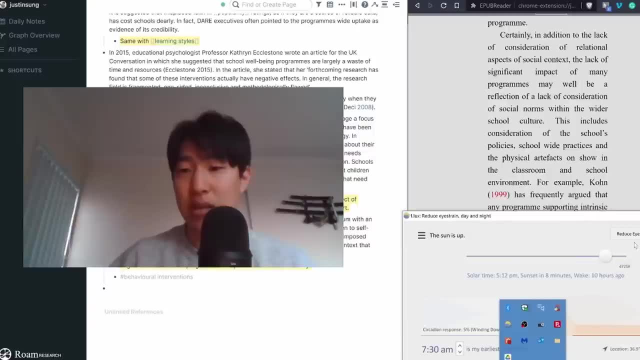 more energy and preserve my reading stamina. And the other thing is just, I set the background of this to a gray and I've got, you know, I've got a little bit of a black and a little bit of a flux turned on at the moment, with reduced eye strain turned on, And that just allows me to.